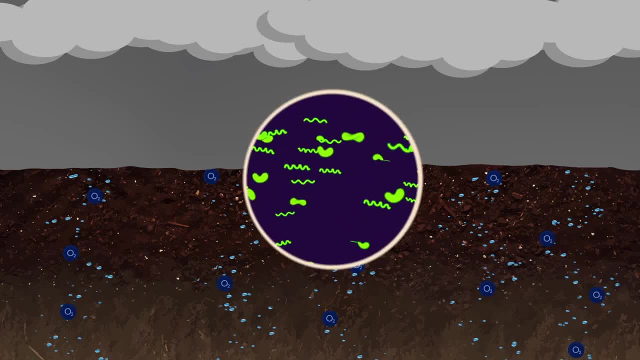 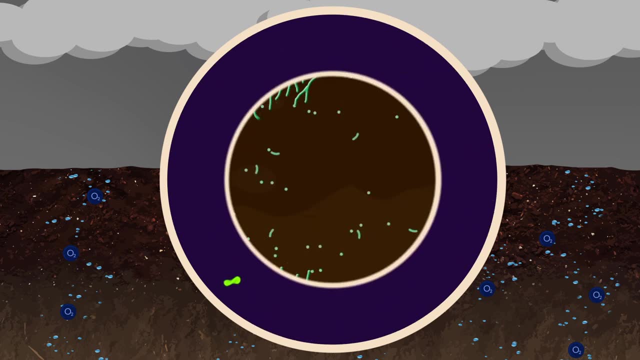 conditions. This is crucially important, as the majority of disease-causing microbes cannot operate in oxygen-rich environments and they are forced to shut down. Meanwhile, beneficial microorganisms thrive in oxygen-rich environments. Water droplets are held in the numerous cracks. 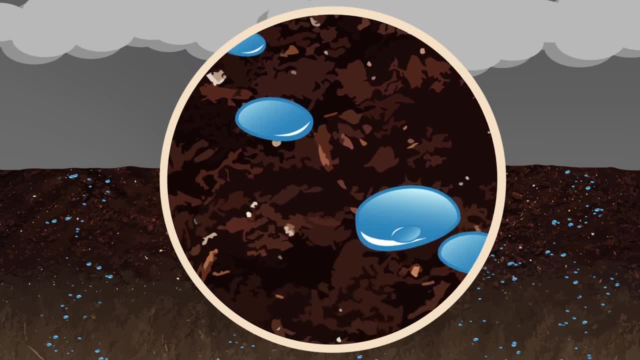 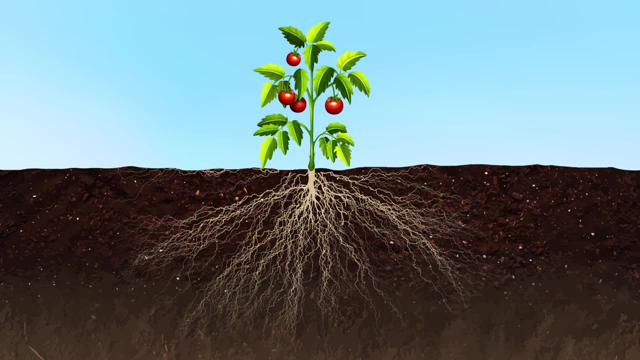 and crevices and in organic matter for long periods of time, thus increasing drought resistance. Good structure allows plant roots to move effortlessly through the soil profile without having to work hard against compaction layers In soils where good structure has not been. 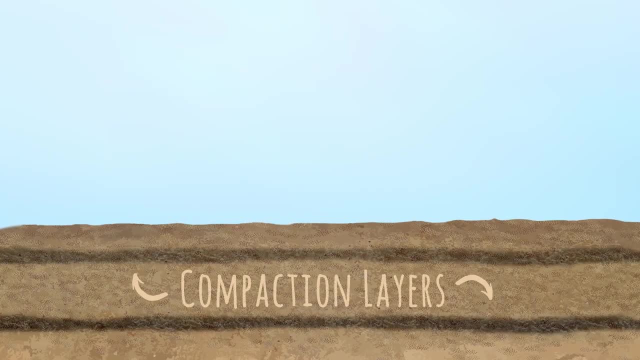 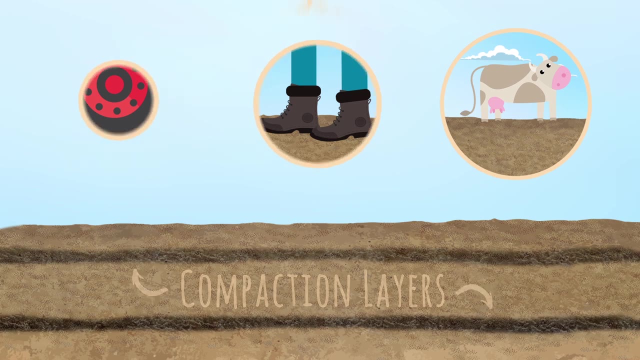 built by beneficial microorganisms. compaction layers are easily formed by vehicles, By human and animal traffic, and where the soil surface is left bare by rainfall. Compaction layers force plant roots to grow sideways, limiting their access to nutrients and water. When plant roots break through compaction layers, they encounter anaerobic or low-oxygen conditions. Those are occupied by anaerobic microorganisms which produce highly acidic compounds. Roots cannot survive in such conditions where the pH can be lower than 4.. 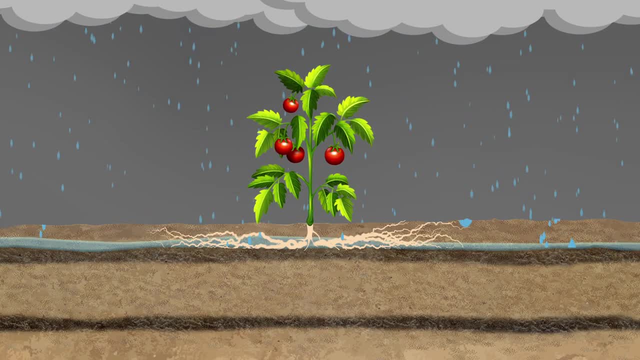 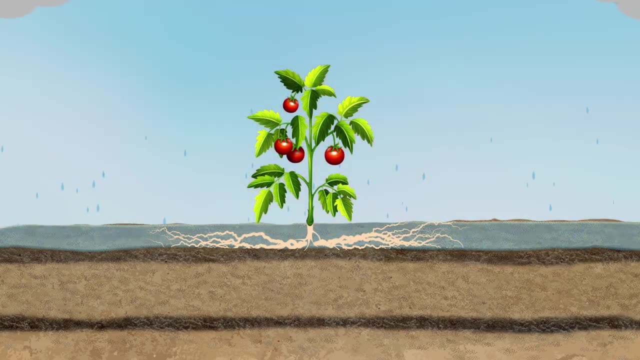 When water flowing through a soil meets a compaction layer, it is possible for the soil to break through. It can't get through, and so in heavy rain this can result in a saturated layer of soil sitting on a hard compaction layer. If there is an incline, the top soil 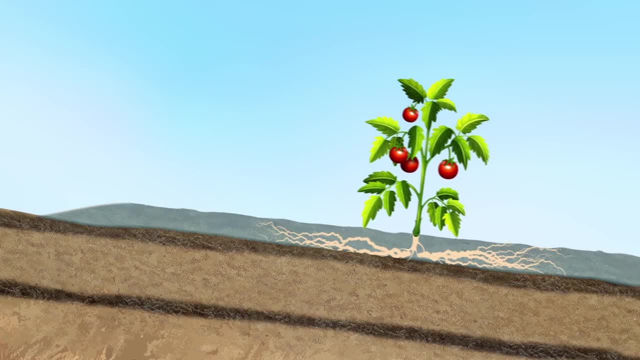 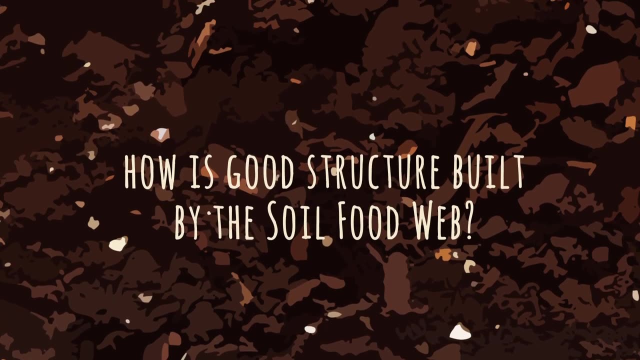 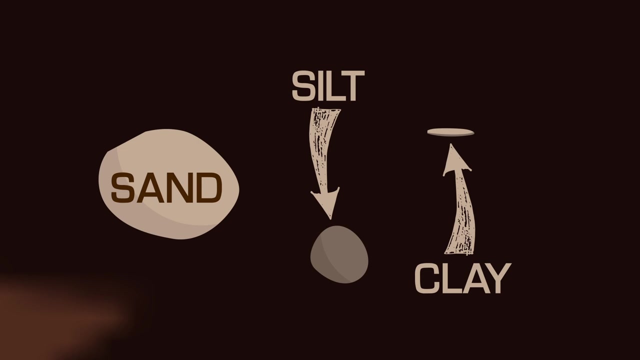 can start to move, resulting in a landslide. This type of soil erosion is a big problem in many places around the world. So how is good structure built by the soil food web? Well, this depends on the type of soil we're dealing with. The terms sand, silt and clay describe the size of the soil. 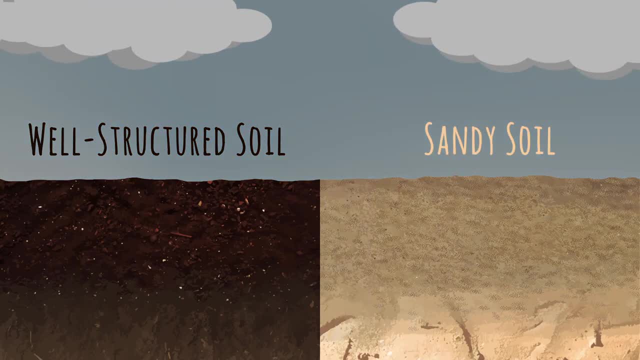 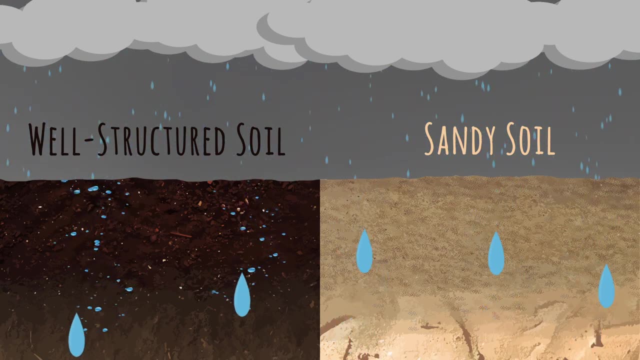 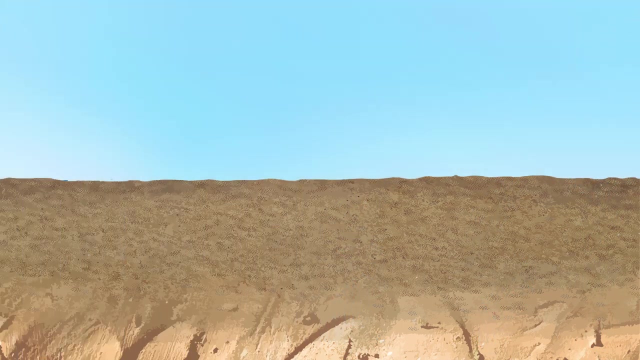 mineral particles. Sand particles are relatively big, and so are the spaces in between them. Water quickly finds its way through the gaps and not very much water is retained, especially if the organic matter content is very low, as organic matter can absorb huge amounts of water, So sandy soils tend to be very dry. 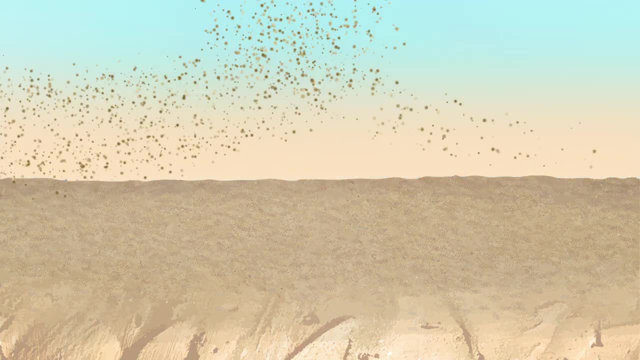 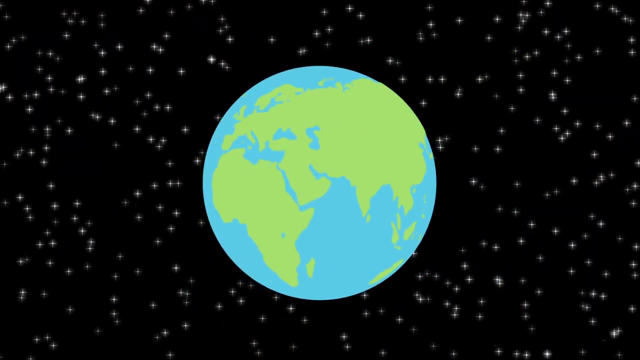 and are prone to wind erosion, which is the process by which the top soil is blown away and lost. Soil erosion is a serious environmental problem and poses an existential threat to humanity. as we only have around 60 years of top soil left in the world. Soil erosion is 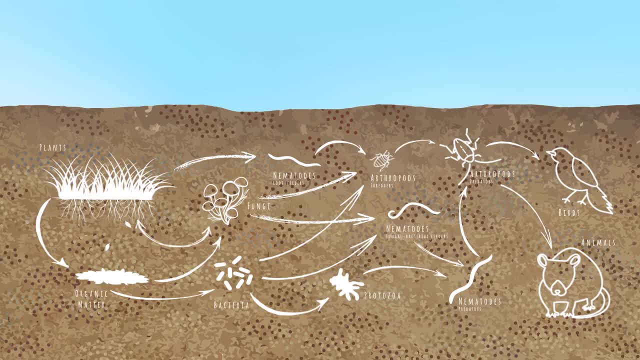 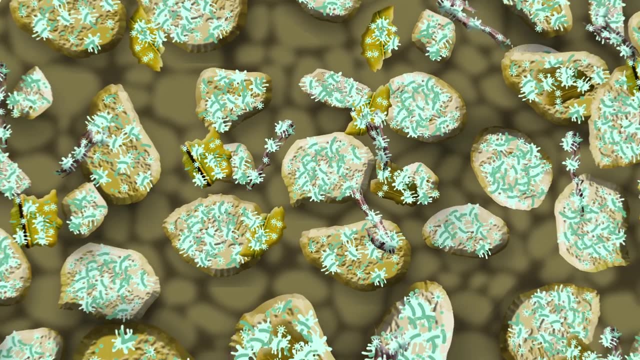 a major problem in many places around the world, according to recent estimates. With the soil food web in place, the picture rapidly changes. Beneficial bacteria produce sticky compounds or glues which make it easy for them to adhere to the surfaces of organic. 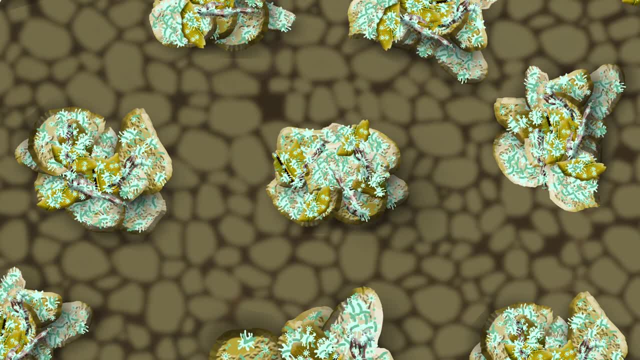 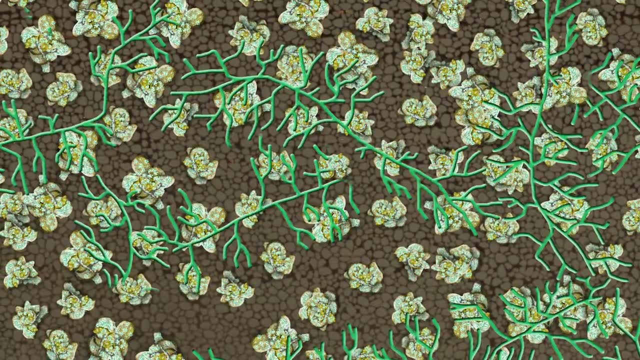 matter and sand particles. These particles then adhere to one another, forming microaggregates. Notice how, as things clump together, small spaces are created around them. Fungi also produce some glues, and their long, narrow tube-like structures act like ropes tying. 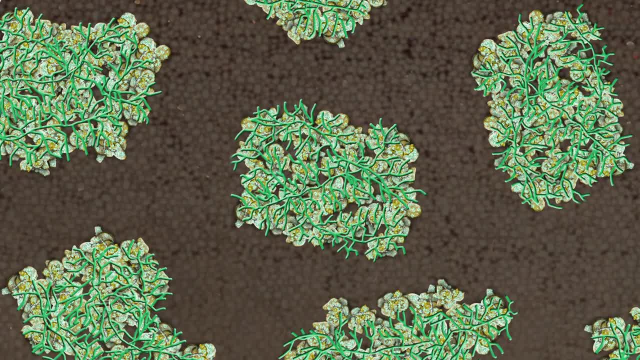 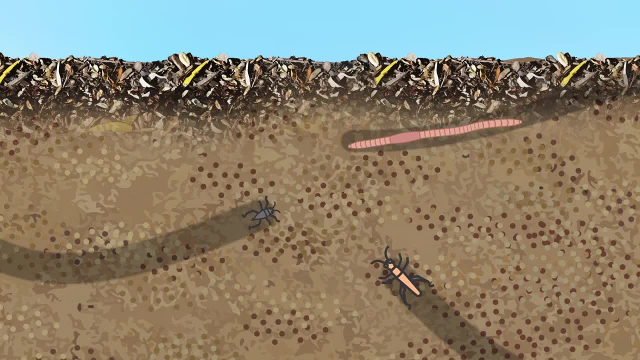 together the microaggregates to form macroaggregates. Now even larger spaces are formed in the soil structure. When microarthropods, earthworms and insects burrow through the soil, they create even larger spaces, like tunnels. 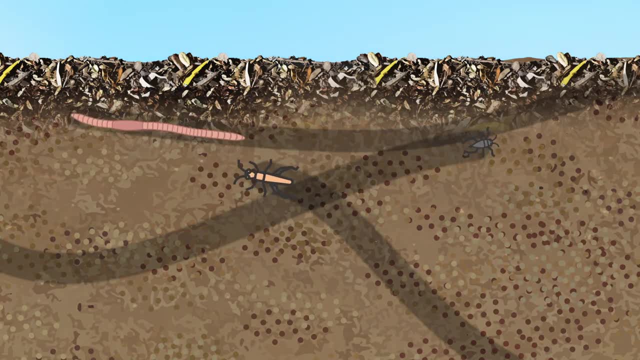 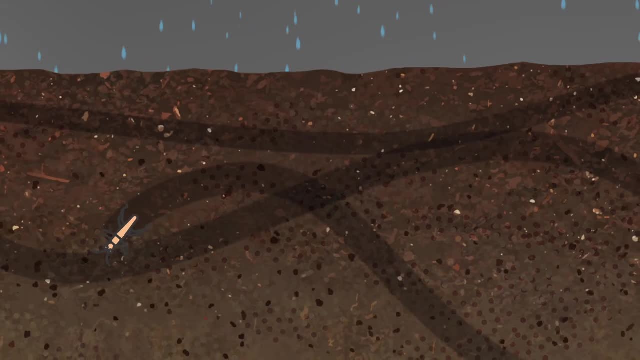 All the while, the soil food web is increasing soil organic matter in the soil profile By decomposing the surface litter into humus and transporting it deeper and deeper into the soil. soon you can dig down and discover layer after layer of dark, chocolate, brown soil. 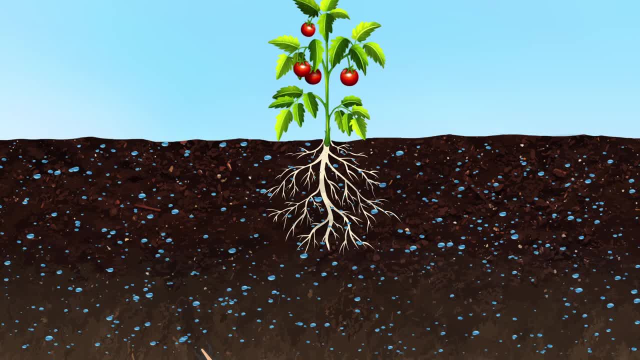 where there was once only lightly colored sand. The result is a structure that will hold water for several months after the rains have stopped, making it available to plants in times of drought. Roots are able to dig much deeper and to access more water and nutrients. 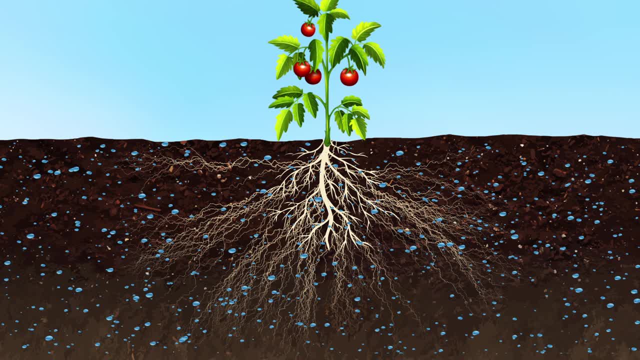 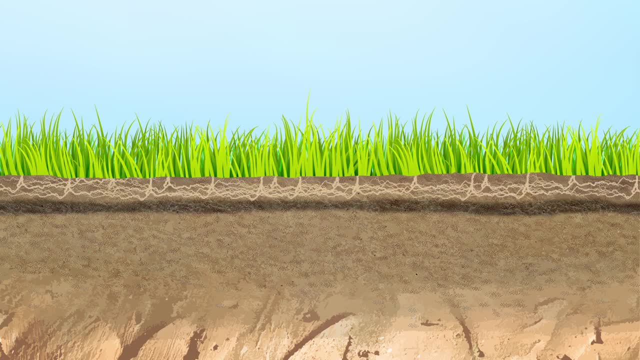 in parts of the soil that were never available to them before. In essence, the subsoil has now become topsoil. Dr Ingham and her team have worked on landscapes such as pastures, turf lawns and golf courses. 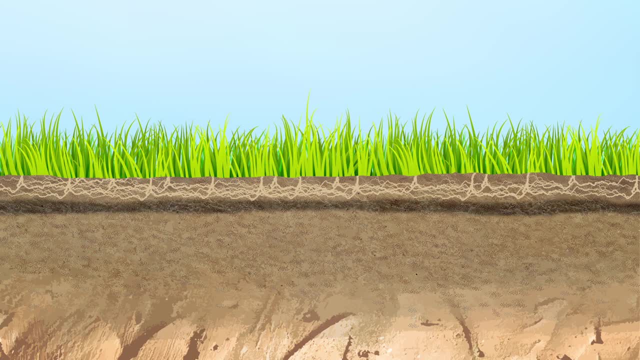 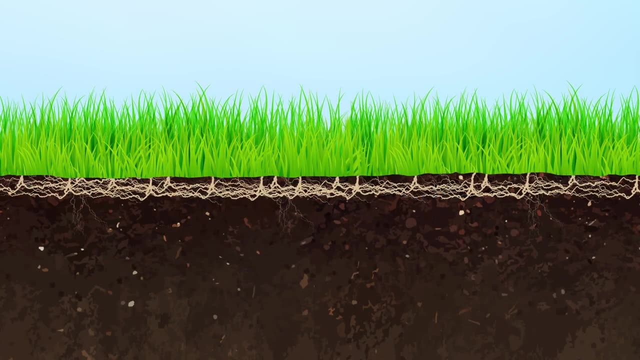 where the grass roots were only able to grow an inch or so into the soil because of the presence of compaction layers, In just a few short months after the soil food web is restored, those same roots are able to grow more than three feet deep. 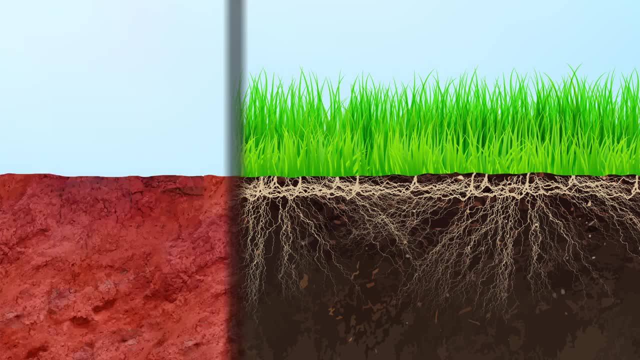 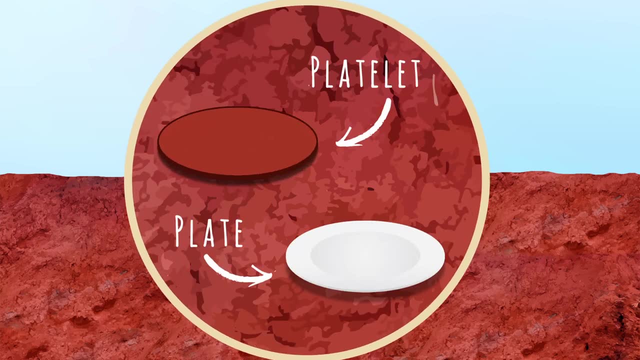 accessing more water and nutrients than ever before. In clay soils, the problems are a little different. Clay particles are often referred to as platelets, as they are kind of round and flat like the plates you have in your kitchen. Without a balanced soil food web, 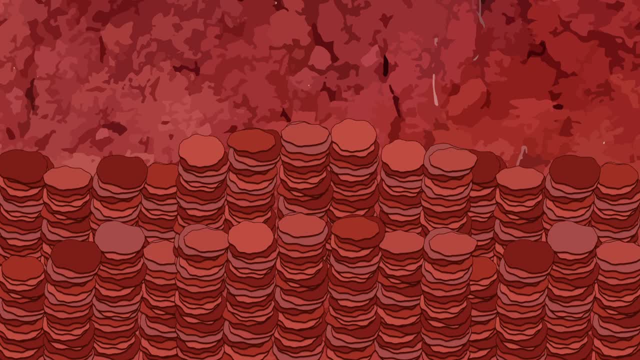 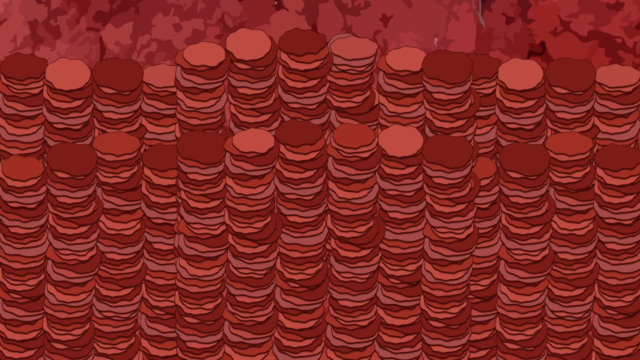 these platelets get stacked up on top of each other, forming very tightly compacted structures. Compaction layers can form very easily in clay soils. The solution to this problem is finding a way to get those clay particles to stop stacking. This can be achieved by a process called flocculation. 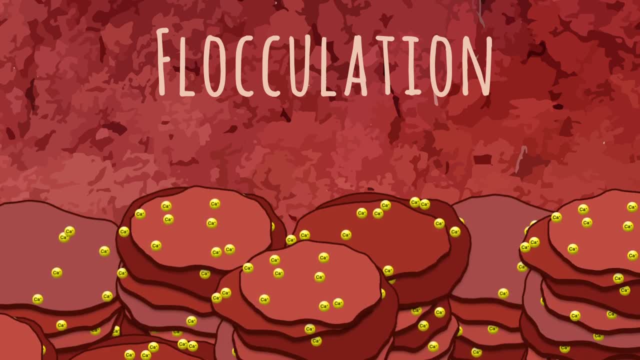 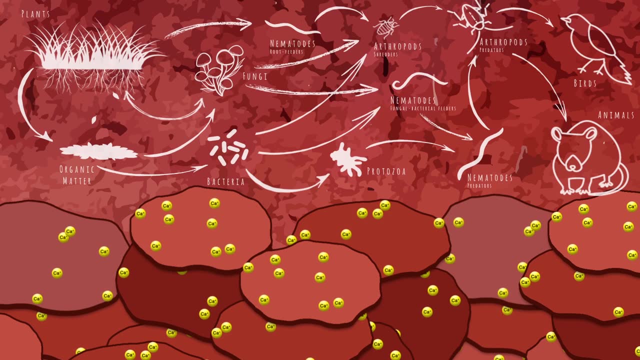 Flocculation occurs when sufficient positively charged calcium ions are present on the surface of the platelets. This results in them repelling each other, just like magnets do. when their poles are aligned, The soil food web increases flocculation, and once this is achieved, structure can be built.